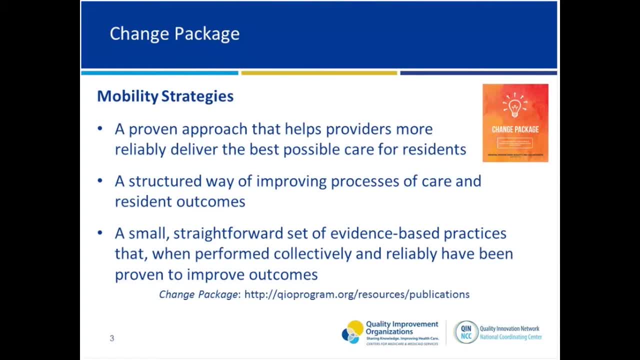 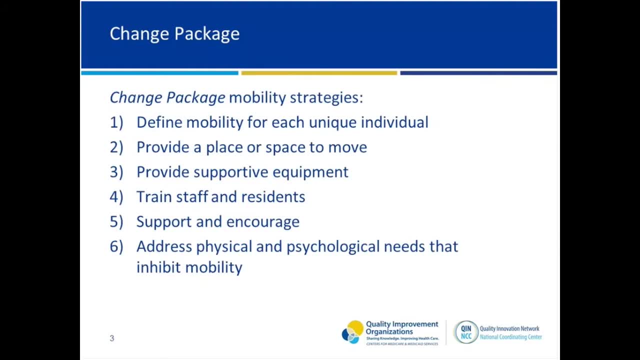 specific action items that can be implemented in your organization. Copies of the change package are available at the website. listed on this slide, You ll see six strategies from the change package: mobility bundle. Within each strategy there is additional detail that will help to implement the strategy. Please refer to. 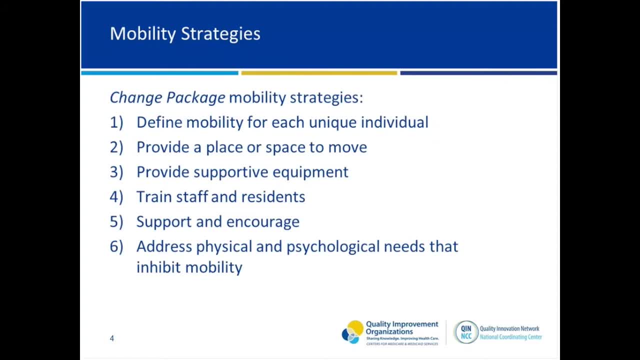 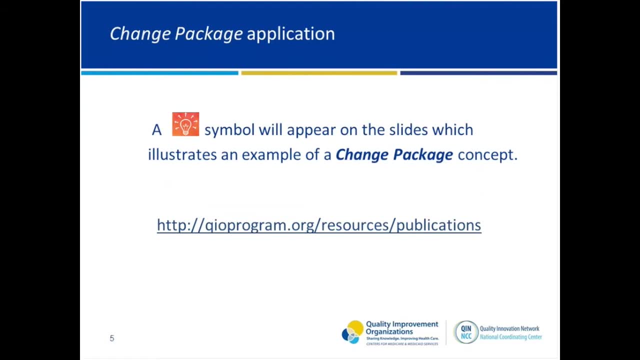 the change package mobility bundle for details of each strategy listed on this slide. Thank-you. You will also note throughout this presentation a lightbulb symbol with numbers listed behind the symbol. This symbol and its following number corresponds to an example of how a specific action item. 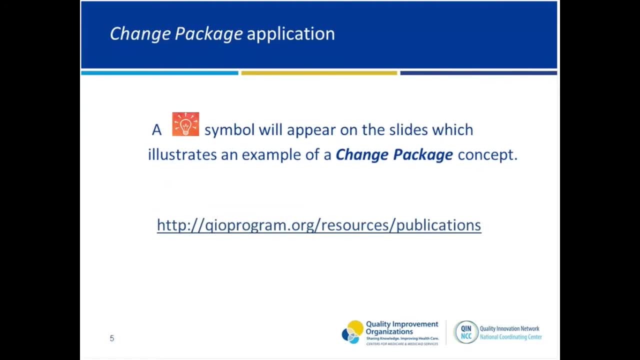 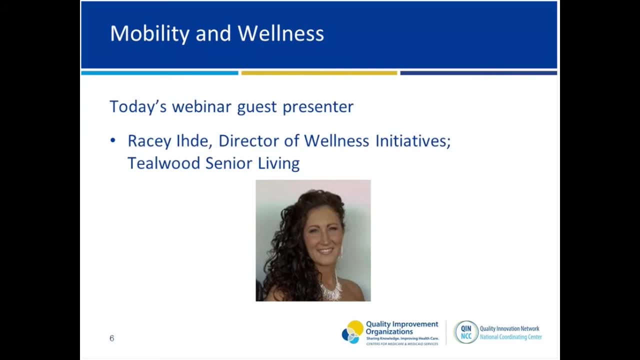 from the change package is being applied. I'm very pleased to introduce Racy Eide, Director of Wellness Initiatives and a Wellness Consultant with Tillwood Senior Living. Racy will share information about a recent quality improvement project that was initially implemented within a collaborative of 11 Minnesota nursing homes. 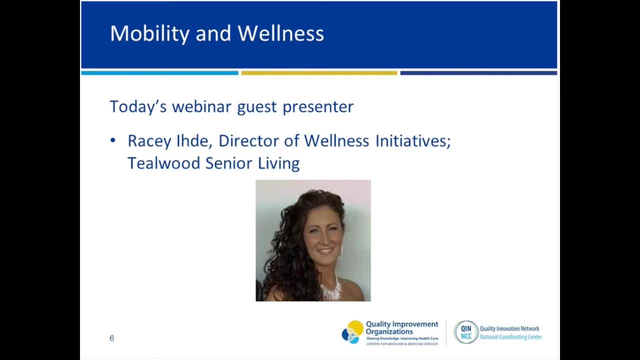 The program had such positive outcomes for residents that it was standardized throughout the entire Tillwood organization of more than 40 nursing homes, assisted living and memory care facilities in communities across four states. Racy is a leader in the area of exercise and is passionate about keeping people moving. 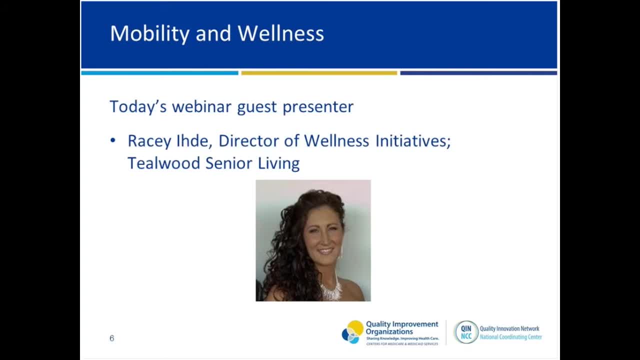 in order to reach their goals. She is a certified personal trainer with an additional Senior Specialty Certificate. She has been working with older adults for about eight years and in the wellness industry since 2006.. She holds a Master's Degree in Human Services and a Bachelor's Degree in Psychology. 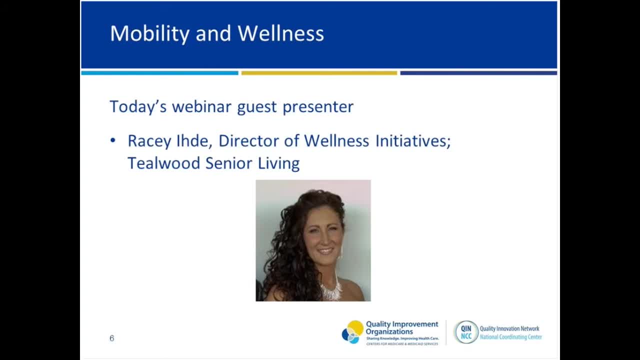 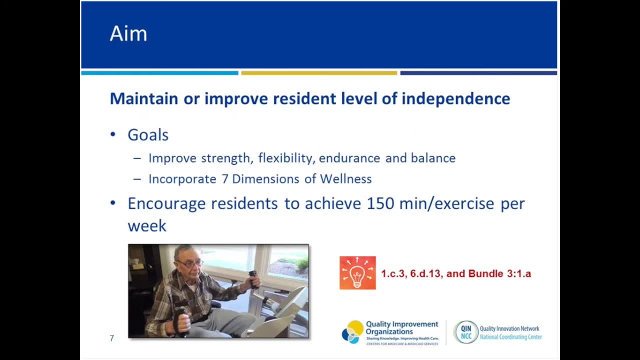 Racy will describe for us Tillwood Senior Living's physical activity program and will also hear from residents that have participated in their program. Welcome, Racy. thanks for joining us. I am anxious to hear about your physical activity program and goals. Ultimately, we would like to assist our residents to maintain or improve their levels. 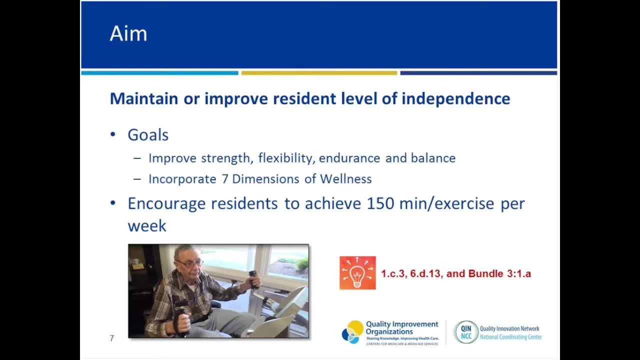 of independence, And by aiming for this, we understand that it is a key concept in ensuring quality of life as well. We really have a couple different direct goals. We focus on improving strengths, flexibility, endurance and fitness. We also focus on improving physical activity and training. 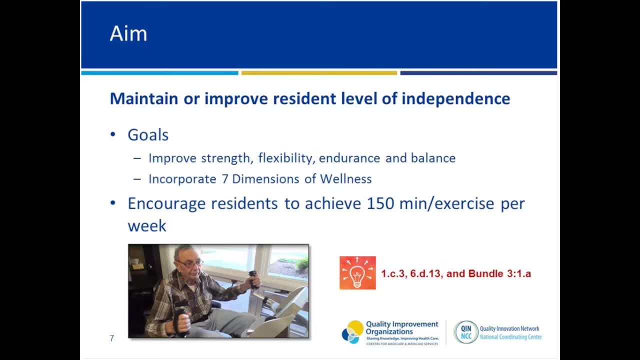 We also focus on improving health and fitness. We also focus on improving physical activity and training balance, along with incorporating the seven dimensions of wellness. In addition, we encourage residents to achieve 150 minutes of exercise per week, and this is recommended for older adults through the American College of Sports Medicine and. 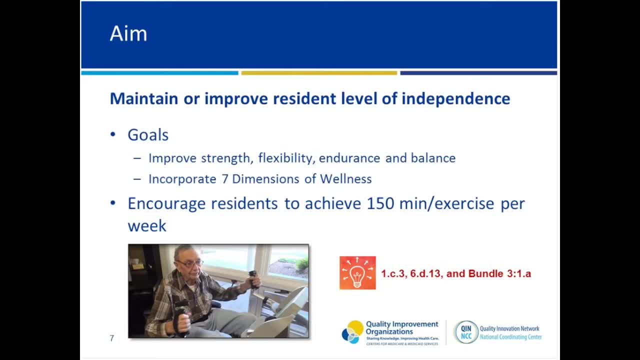 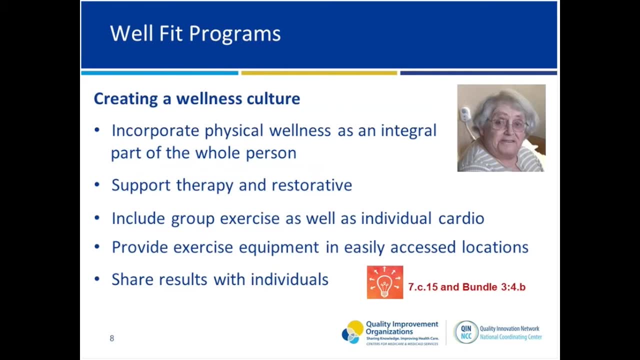 it actually has additional evidence-based research behind it for improving sleep quality. We look at physical wellness as a whole, so we not only support therapy and restorative, but also have created what we call our WellFit program. that includes group exercise and individual cardio In. 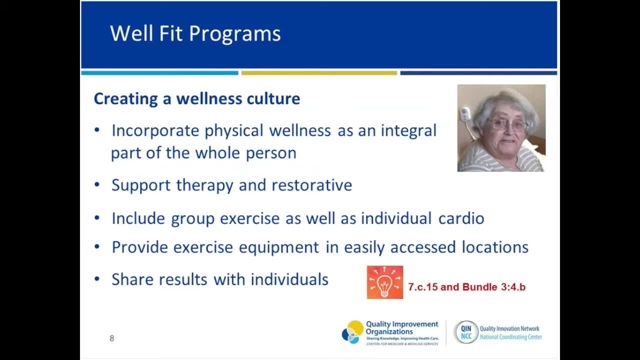 addition, our company aims to establish a wellness-based culture within all of our communities, So an example would be: a piece of cardio equipment is placed out in the open instead of tucked away into a back room. We're also adjusting budgets now to include dumbbells and other exercise equipment and wellness rooms. 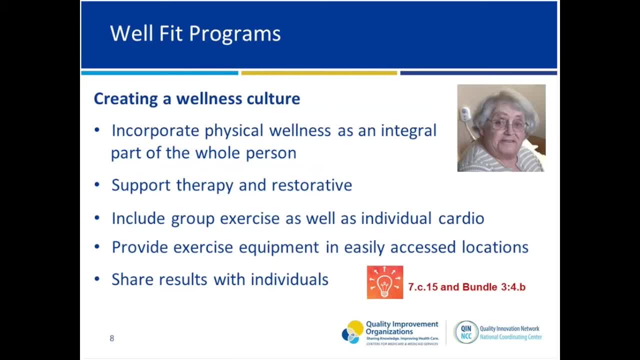 are now a staple within our future building projects, So we ultimately provide the wellness-based culture within all of our communities. We also constantly remind that remaining physically able is important for the aging population. We definitely share WellFit test results with each individual resident as well. So by strongly believing that maintenance is a 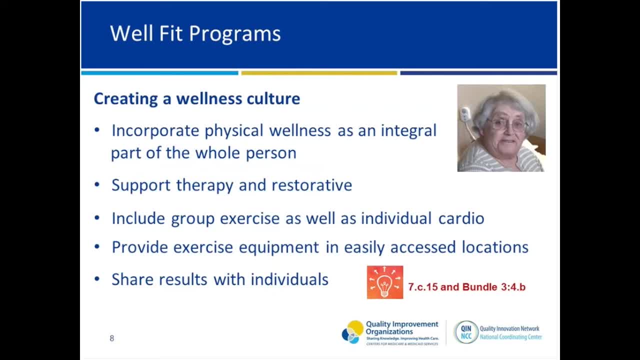 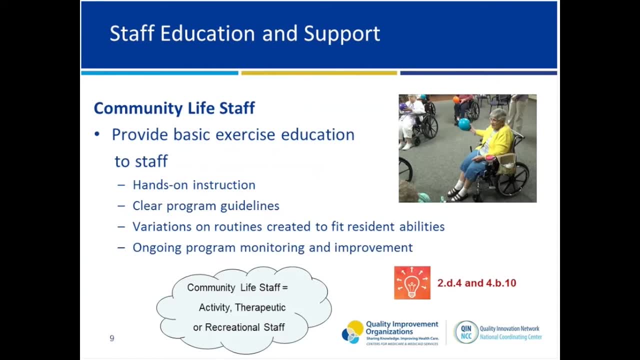 success. we help to encourage more of the participants to stay active than those that just improve. For the most part, our Community Life staff run our WellFit programs. We offer initial and annual education on basic exercise knowledge, as well as hands-on instruction on how to properly teach group exercise classes. 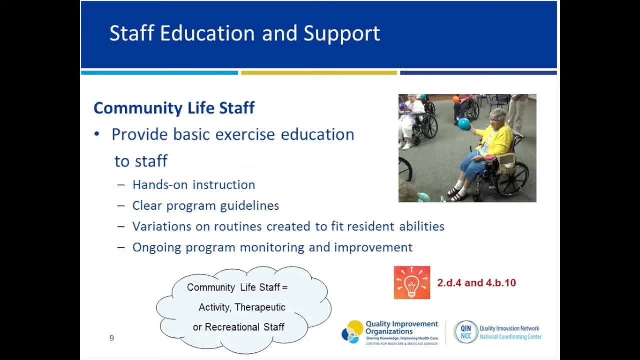 Guidelines of the programs are clear and concise, and the exercise routines require specific concepts that need to be included. However, stats are taught variations within each routine so they can properly adjust to fit to the ability of the population they are leading. Those programs are then. 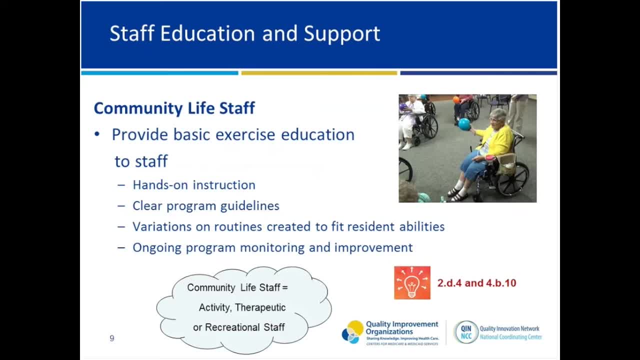 monitored on a monthly basis by wellness consultants and suggestions for improvements are given accordingly. In particular, we give the community a role to play in improving their well-being and personal well-being. We also educate other departments on the importance of keeping residents as independent as possible. 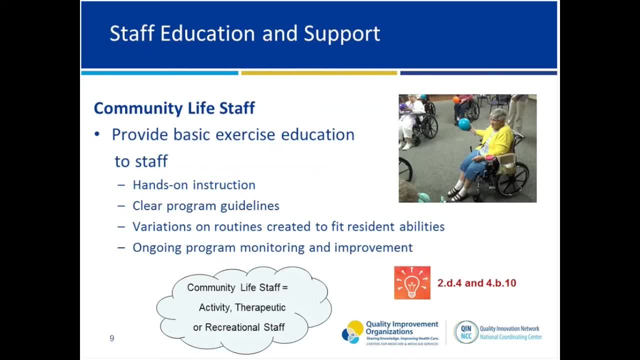 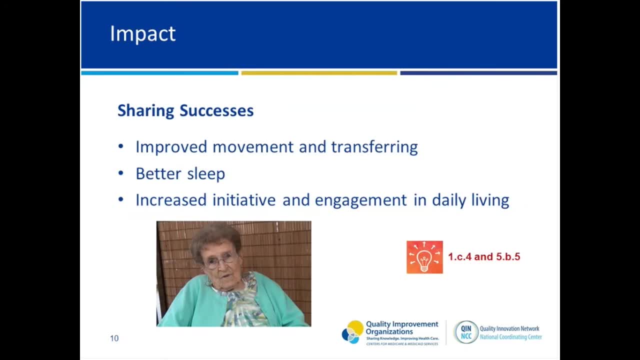 So we offer research-based techniques and approaches within our training modules for differing departments. I would like to hear more about your physical activity program. What successes would you attribute to your program? There have been various success stories in relation to mobility within our communities. 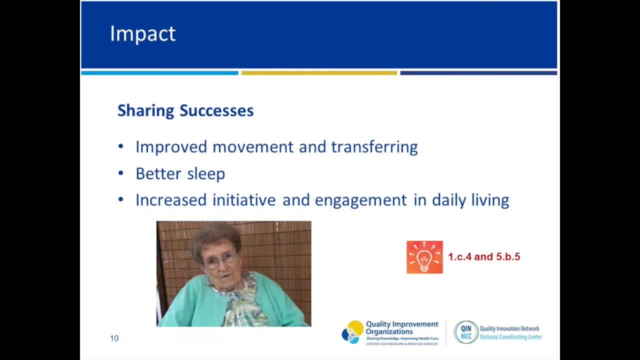 We actually make it a point to share our successes when we get all of our staff together at our biannual meetings. Some staff have shared. an example would be one woman who exercised on a regular basis stated her excitement for now being able to transfer herself into the salon chair at the beauty shop. 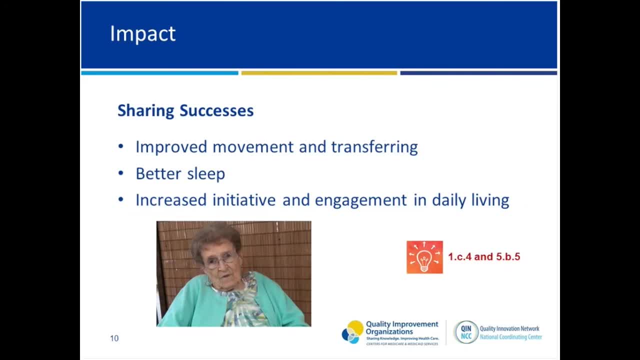 So you could just see it in her face at how proud she was to say: I can do it myself. So that was a really big success for her, improving her quality of life. Others that have participated have commented that after only three months of participating, 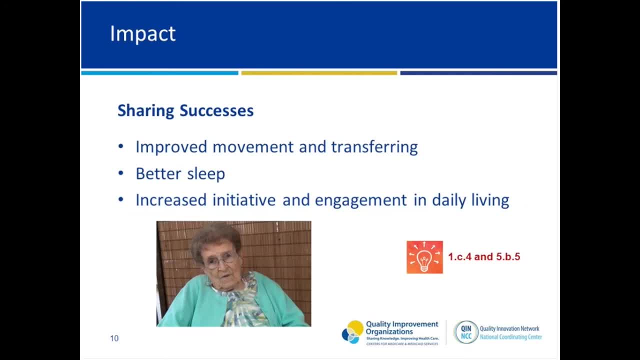 within the WellFit programs, they stated, I have been sleeping better at night and I can move my legs, feet and ankles more than I could in the past three years. It seems, too, that our WellFit programs have become a gateway that individuals who participate 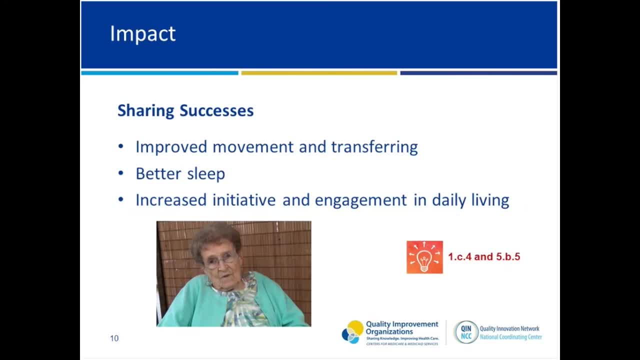 soon begin to join into other things. It ultimately encourages an active lifestyle. So staff have noticed within that active lifestyle improvements in transfers, residents doing more for themselves, Residents taking the initiative during ADLs initiative in assisting with cares and taking more charge of their overall well-being. 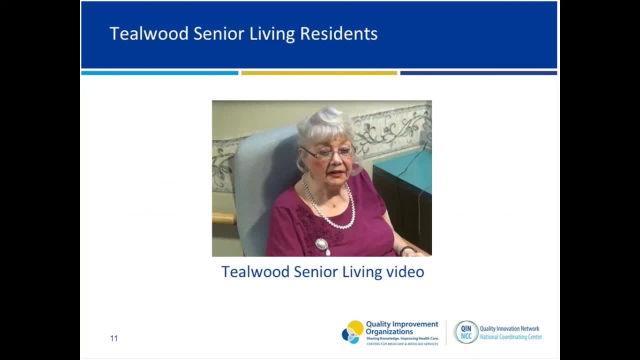 Racy, it's been great to hear about your physical activity initiatives. Let's hear from residents who have participated in Teal Woods Physical Activity Program. Now tell us about their experiences of increasing their physical activity. Yes, it's been helping me. 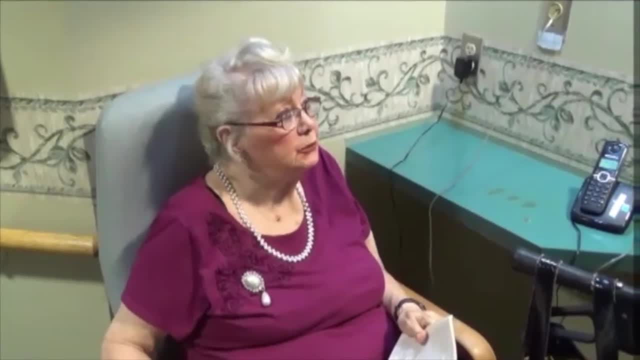 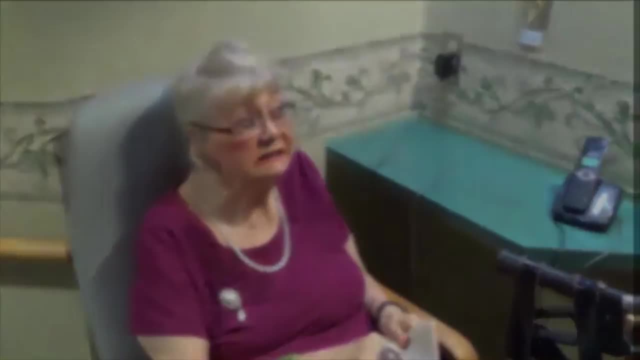 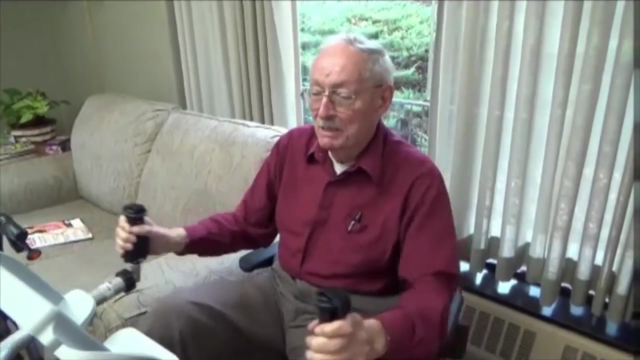 I can stand up. You know where you use the arms, then you use your knees, And I think I've lost quite a bit of weight too. You do, Yes. Well, I suppose it keeps my legs going. Well, it keeps me going better. 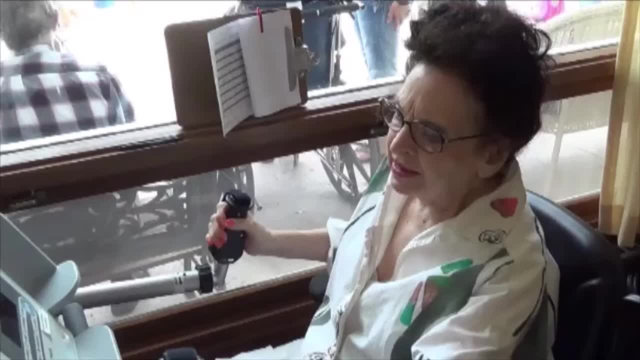 If I just sit around and do nothing pretty soon you can't do much. I think it kind of takes the kicks out of your muscles and stuff first thing in the morning and everything if you get on it or any time during the day. 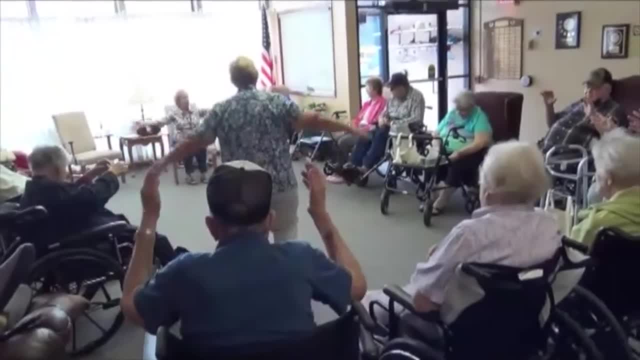 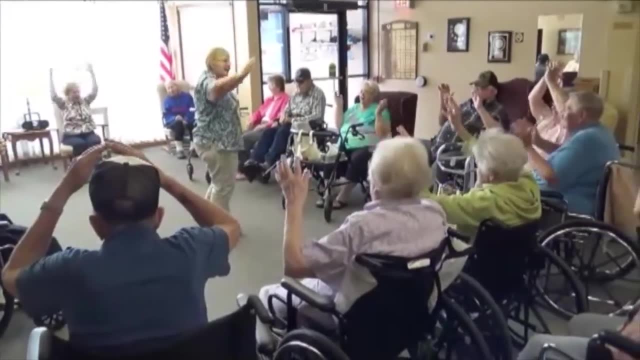 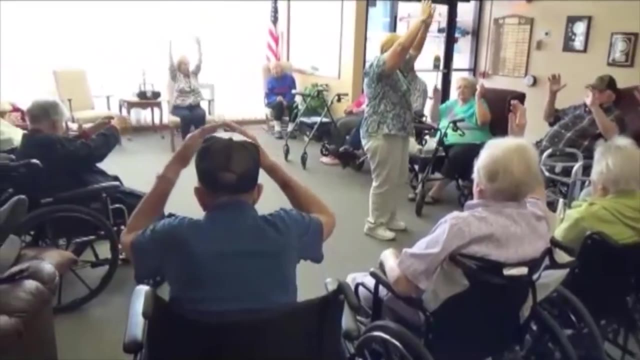 And it kind of relaxes you. Yeah, Hey, hey, hey, hey, hey and down. Hey, hey, hey, hey, hey and down, All right Down. Oh, oh, oh, oh oh. 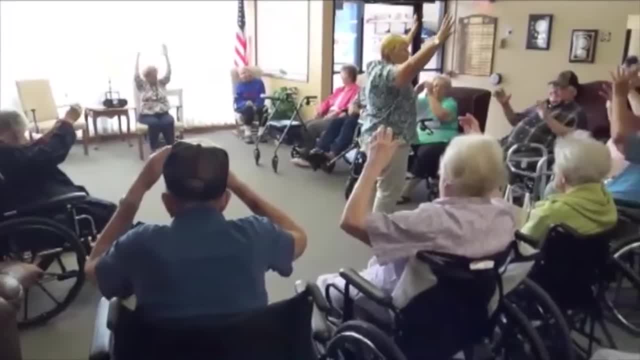 Okay, and you, You, you, you. Well, it kind of keeps your strength up.